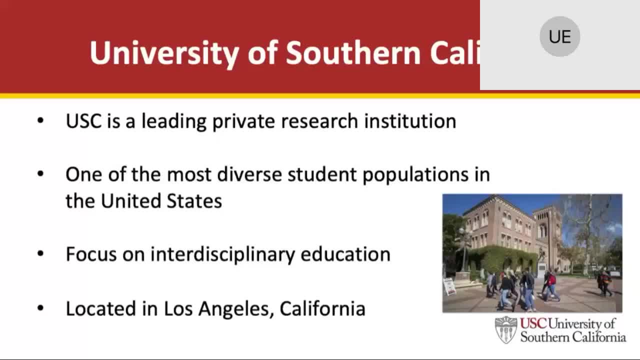 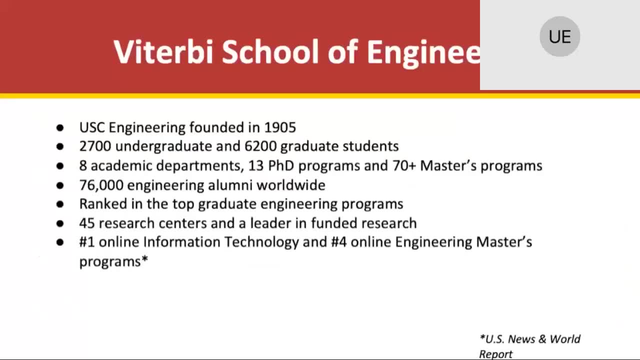 Okay, so it's a very graduate student friendly population. Within the Viterbi school of engineering, we actually have a similar ratio as well, that we have more graduate students than undergrads. you see, right there Within the engineering school, we have 8 academic departments. 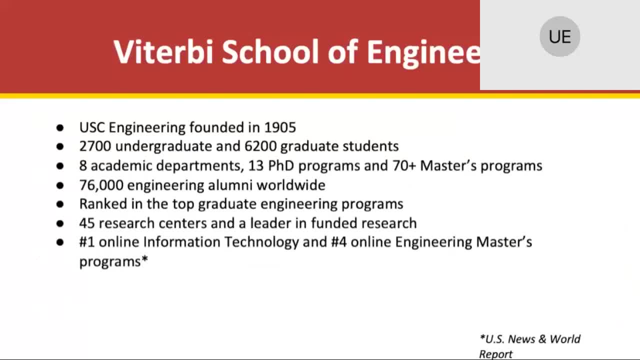 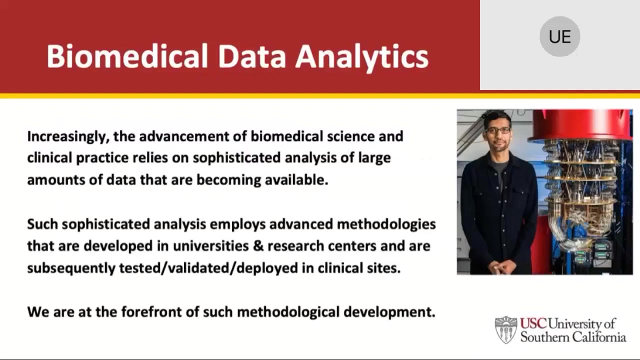 13 PhD programs and over 70 master's programs. So at the master's level you really can specialize in a particular area, such as what you're here to learn more about today: the master of science and biomedical data analytics. So, without further ado, I'm going to hand off the access to Dr Marmorella and 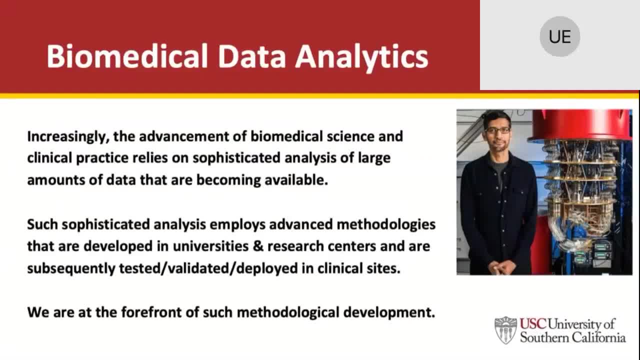 make him a presenter So he can speak about this program that you're all joining to learn more about. Thank you so much. Yes, thank you. I trust you can hear me. Good evening everybody. I'm glad to be here with you and to try to give you some information about the new master's program in biomedical data analytics. 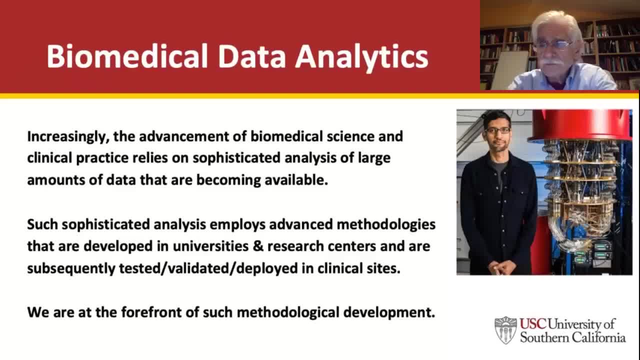 Then I can see that we have 5 participants And I can say not participants and I will tell you a few introductory remarks and then I would like to solicit your questions and comments, because that may be More useful to you to direct me with your comments. but let me go down this 1st slide. I trust you can all see. 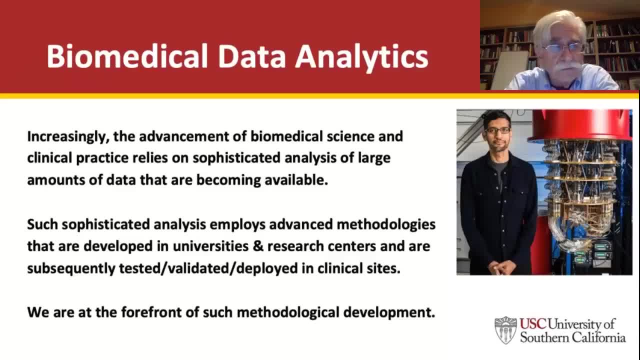 And it basically states the fact that we, More and more The advancement of medical science and clinical practice relies on the sophisticated analysis of large amounts of data, and such large amounts of data are becoming available more and more So because we, of course, the advance and improve the means by which we collect data. with acquired data, 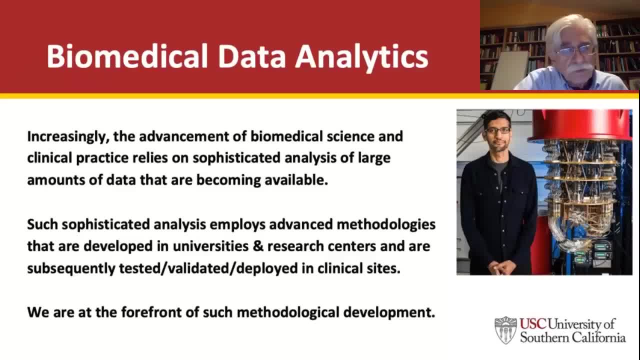 Therefore, the direction of the future is clearly the direction where we will have to analyze Large amounts of data That will become increasingly available, And do so in a way that we can advance Both the science and the practice of medicine, And in that I include, of course, biological sciences and the related practice of, let's say, pharmaceuticals, et cetera. 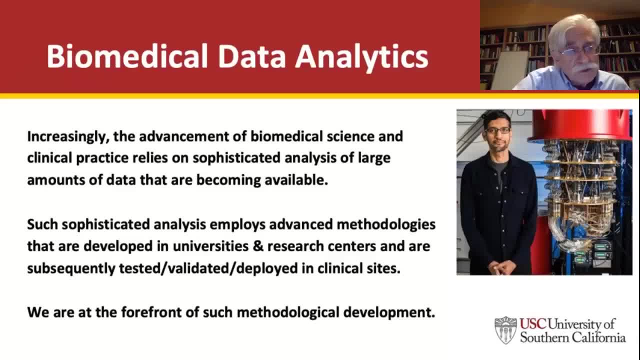 Of course it is obvious that such a Sophisticated analysis- I call it just simply to set apart from the kind of Pretty basic standard type of data analysis that You know you can be exposed in many different programs, Of course is. 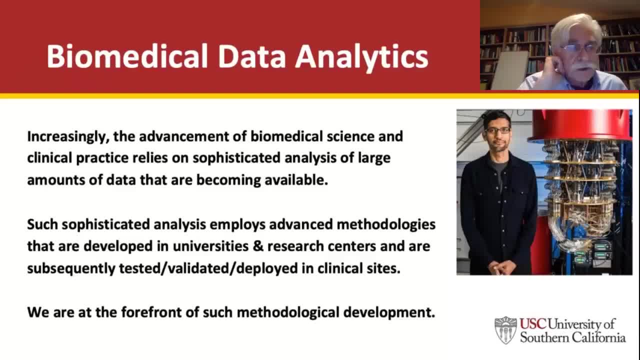 To name an example would be regression, for instance. Regression is extremely valuable. It has paid tremendous dividends. I do not put it down. I simply want to say that it's pretty run of the mill and therefore it's not What I would call sophisticated data analysis at this point in time. 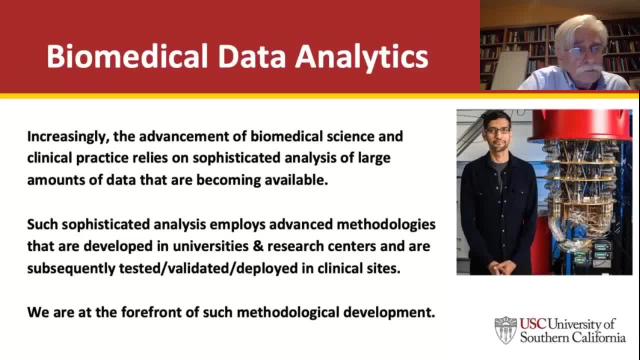 Um. Nonetheless, we can make good use of it in connection with our more sophisticated methods as well. So um the type of methodology we use to achieve this kind of sophisticated, so called analysis Um are developed, of course, in um. 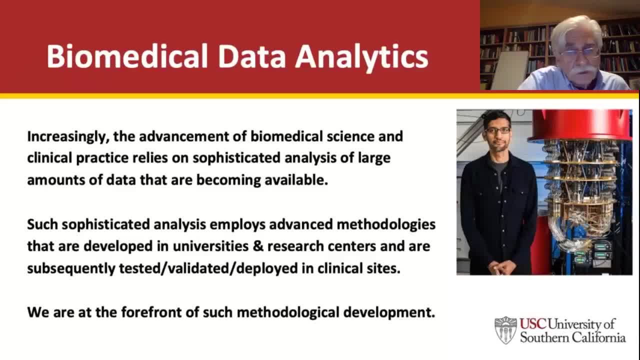 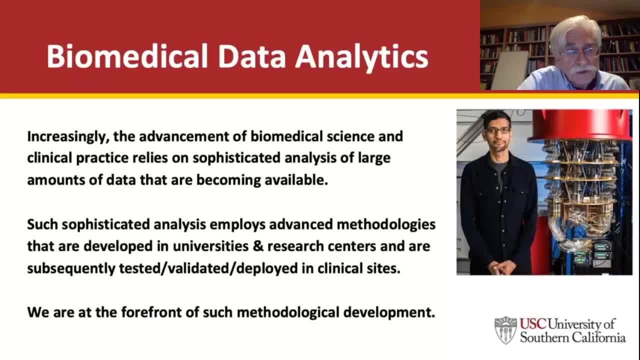 Which is really the primary task of viruses engineers, Um, they are subsequently tested, validated and deployed in clinical sites, And in that process, of course, we have to be Participating, and in a very critical role actually, but certainly we need. 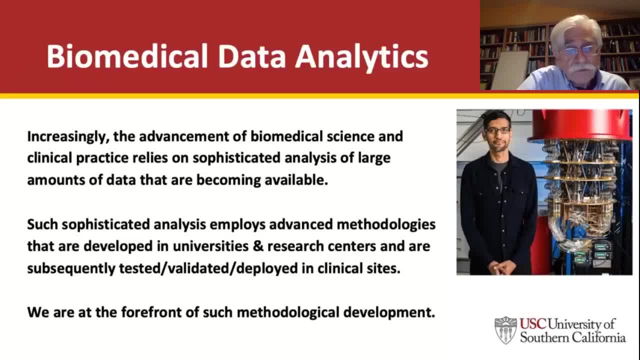 The, the primary involvement of clinicians And uh Um other professionals who give us access to, Uh, the particular domain of medicine that we're interested in, The key takeaways that we believe that in our, Our banner countries, but we are at the forefront of such methodological development. 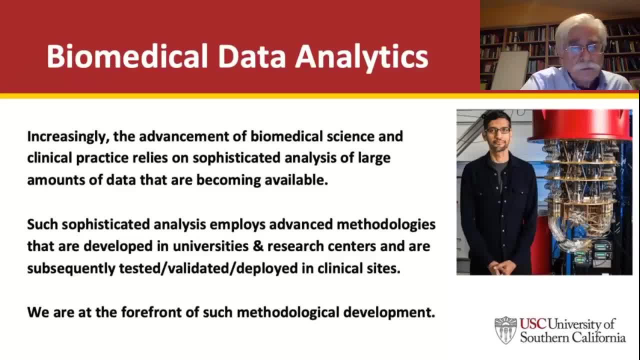 And if you enroll in our master's program, we will, We'll be able to share with you some of this, Uh, so called advanced Those developed, along with some of the methodologies that have been developed in other places. then i should know that the the photo that i have in this slide is not my photo, and i 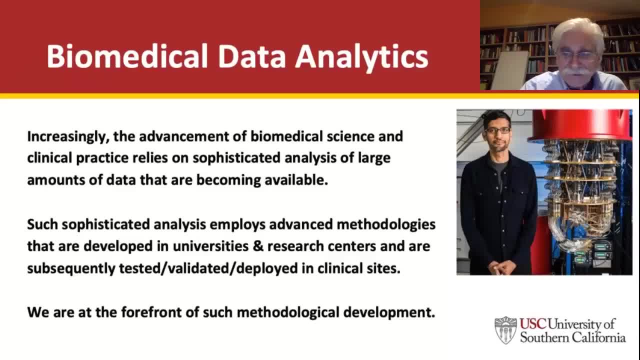 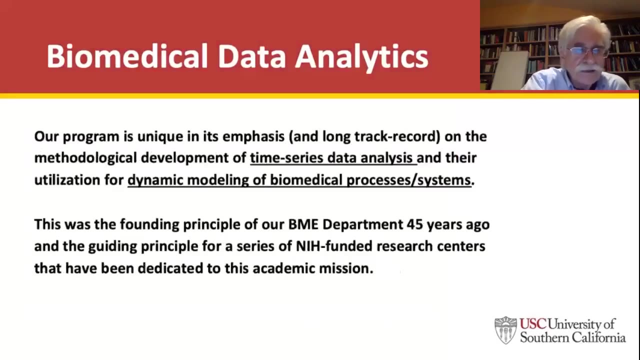 not quite sure how, how it found itself there, but that's quite right at the mind. it looks like rather complicated piece of machinery there, but we don't do complicated pieces of machinery, we just do software. of course you can imagine in mathematics and computational sciences. um, i um going on to the next slide, um, i would like to point out that the program is unique. 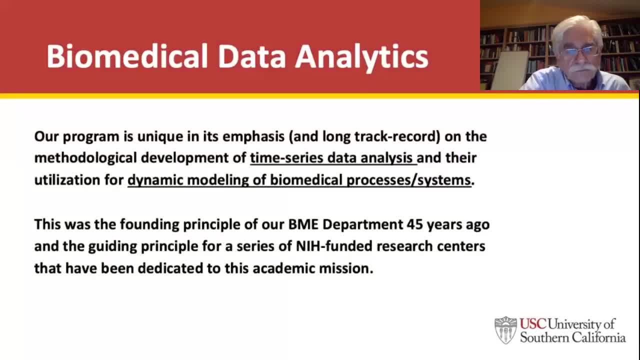 uh, in its emphasis and really long track record on such methodological development, and especially in the case of time series data analysis. i would like to take a few minutes to explain to you a little bit about the methodologies that have been developed in other places, and you know what is the distinction between other types of data and time series data. 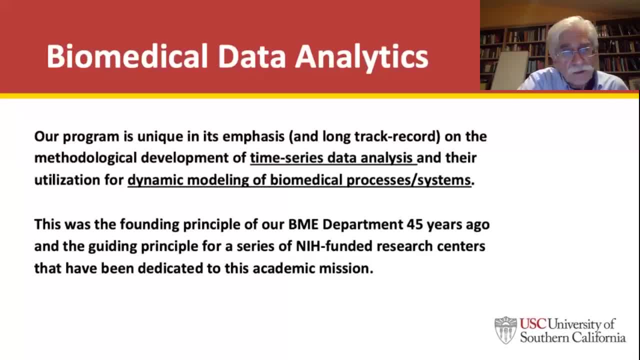 and analysis, as well as the their utilization for what is called here the dynamic modeling of biomedical process or systems. in the types of data that one can collect, of course there are many different types, but in a very broad sense one could separate them in data that are categorical. 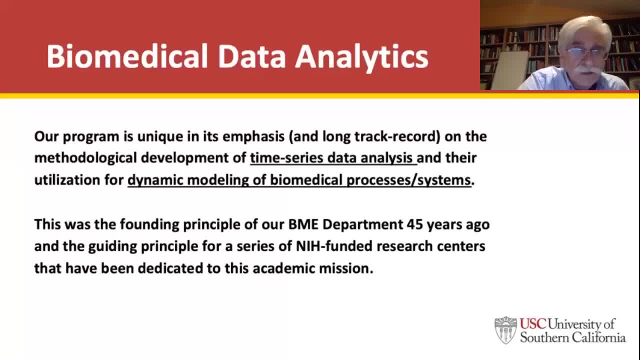 which you collect data of whatever you released in and just make columns of such data in a spreadsheet, let's say, or equivalent Could be also data that you collect in sequence over time by monitoring a specific variable of interest over time, using, of course, the appropriate instrument. 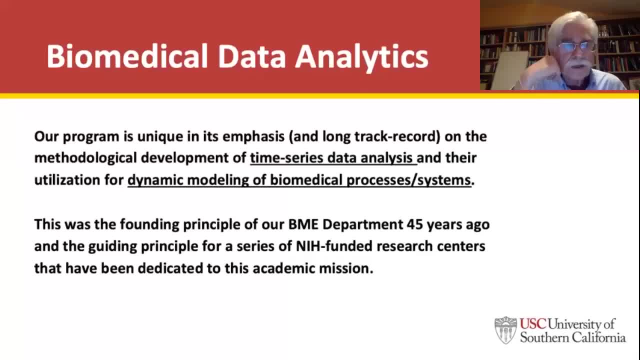 This series of data that we collect over time we call time series data. The analysis of such data reveals the dynamics of the underlying processes that we are observing, And this leads us to the concept of what I have underlined in this bullet. that says dynamic modeling of biomedical processes- slash systems. 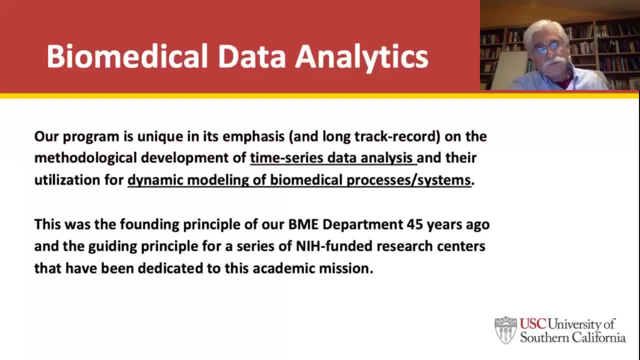 Again, what this means is that, by doing such analysis of time series data, we are able to discover, you know, we are able to discover the kind of mathematical or computational relationships that underline the generation of such data and pertain, of course, 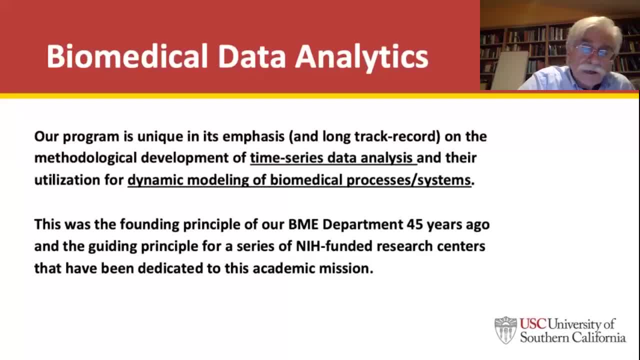 to the system of interest and do so in a dynamic sense, within the dynamics of those processes. To use a very simple example to illustrate this: consider that you have the ability from through could be a single wearable, Actually- to measure the heart rate of a person and also the blood oxygen saturation level. 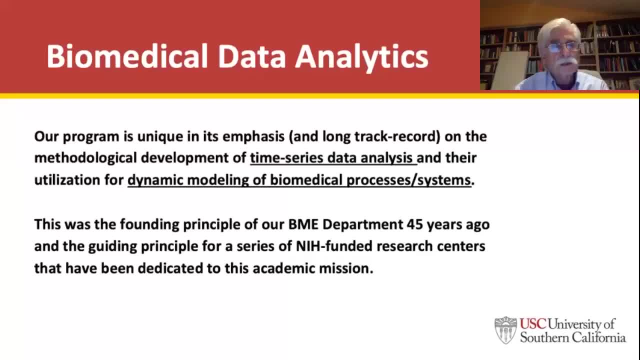 So you have two variables. in this simple example, I'm using heart rate and blood oxygenation. Of course, they both vary all the time in each one of us. By performing the type of Time series and data analysis I'm referring to, what you can do is you can extract dynamic models. 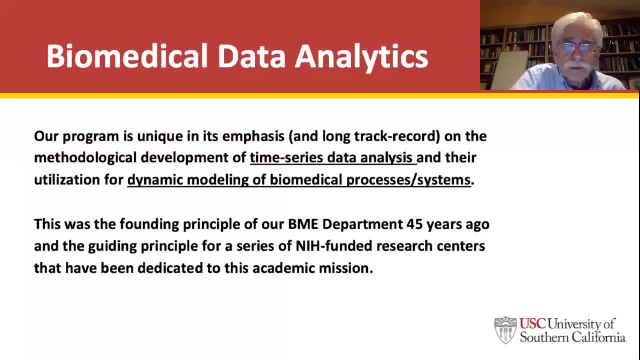 of the relationship, the dynamic relation between blood oxygenation and heart rate That we call that model. dynamic model is really a mathematical or computational relationship between those two variables And that is extracted from the specific data you collect through, let's say, wearable or equivalent. 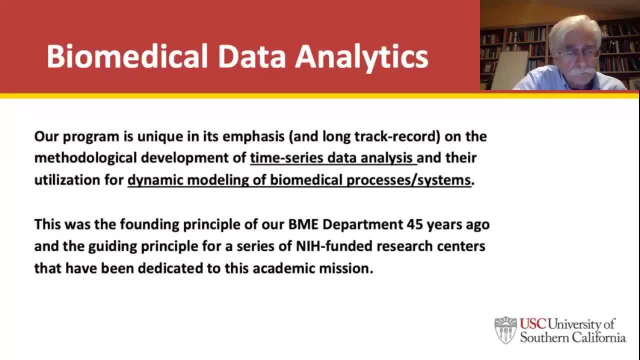 Of course, this can take place in the hospital as well, or the clinic, And that model now has its value in revealing to you the relationship between those two variables. It tells you something about what is going on in your own body with regard to the relationship between those two variables. 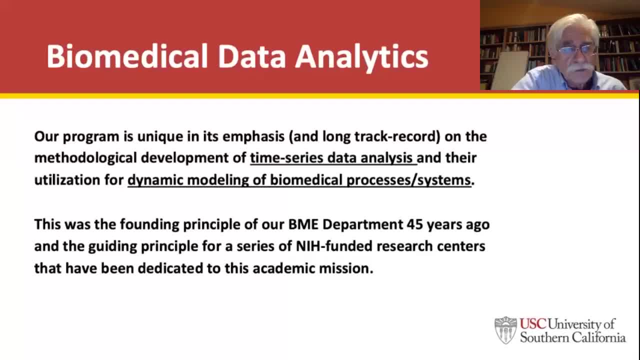 In this particular case, the first thing that comes to mind as an example is the function of the so-called chemoreflex regulation. So the basic physiological reflex we all have in our bodies, And the study of that is of extreme importance in my view. 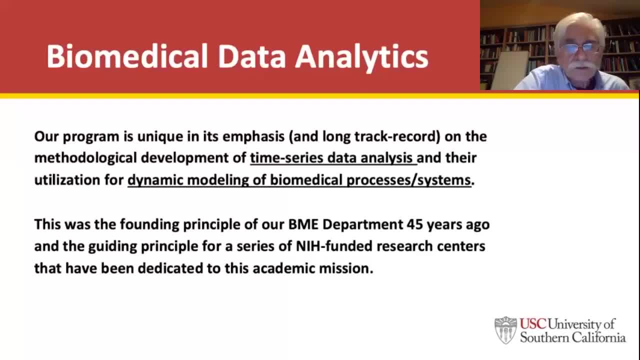 Quite underrated, I have to say, And one of the most common, actually one of the most recent reminders of how important this is- is what you may have read in the media about the severe- some severe- COVID-19 cases over the last few months. 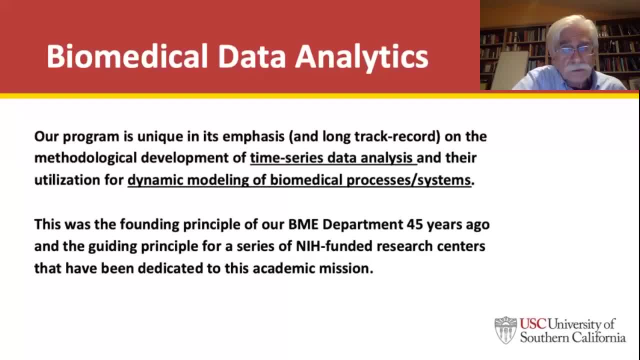 that exhibited very severe hypoxia. hypoxilia, in other words, a severe drop in the oxygen level in the blood of those- unfortunately In patients- without necessarily triggering the normal reflexes that one would expect if the chemoreflex in those individuals was properly functioning. 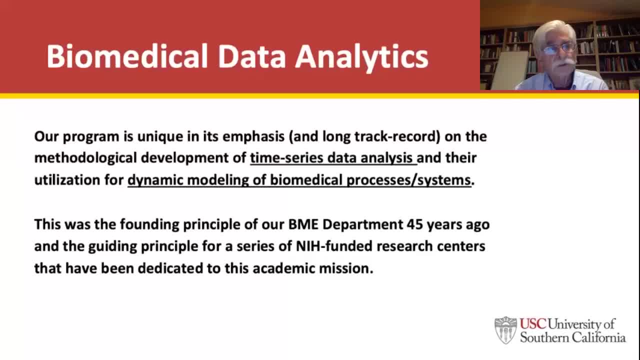 And the probably reflex would be an increase in heart rate and increase in respiratory rate and a few other effects. So I'm just offering this as a quick and simple example of what one can learn It's. I would like to stress that the importance of such piece of information. 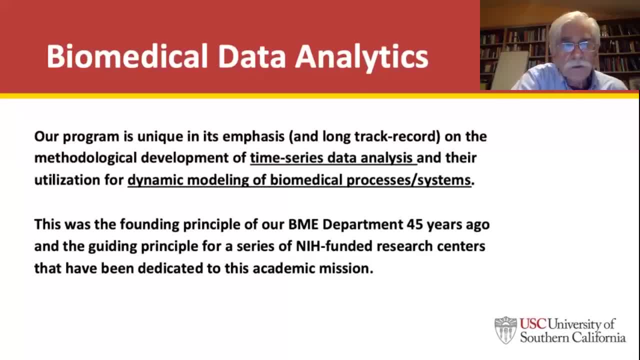 and knowledge is both scientific and clinical. Scientific because it advances our understanding of the systems, therefore builds a foundation for the future of medicine, And clinical because, of course, it can be used potentially to assist the physicians in the clinical setting and, of course, save lives or improve lives. 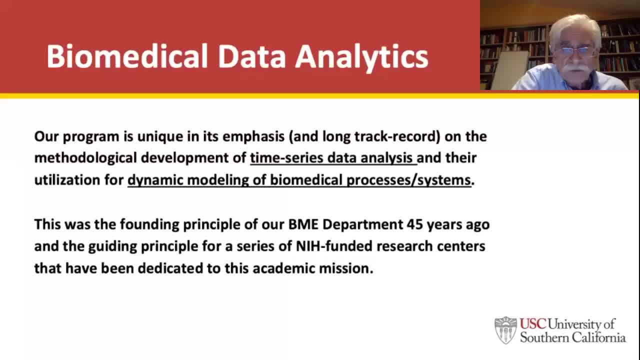 In the short time we have, I think that's one example that is, I think, illustrates the point that I'm trying to make. with regard to dynamic modeling, I'm taking your time and mine to do so, because that's not so widely understood or appreciated. 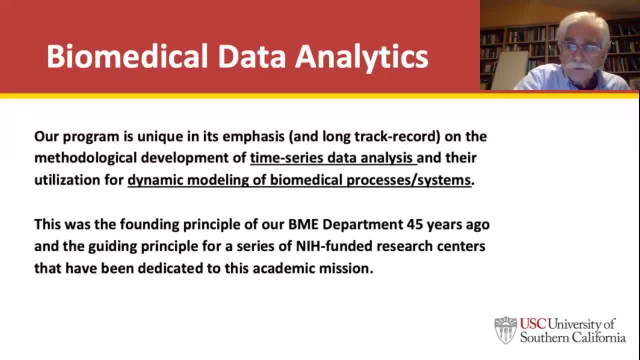 Perhaps I'm wrong, and I would like to have, of course, your feedback on that or questions in a few minutes if you want to share with us. This is what I just described was the founding principal, actually, of our Biomedical Engineering Department, 45 years. 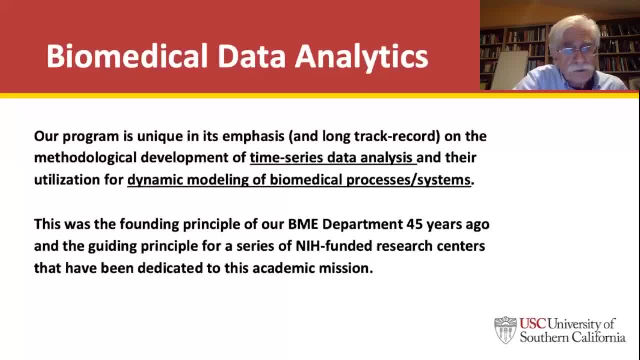 ago And the guiding principal for a series of NIH-funded research centers, one of which I led with Professor Bergenio. for you know, 35 years- a long time- And those have been dedicated to this academic mission and it's a point obviously of pride. 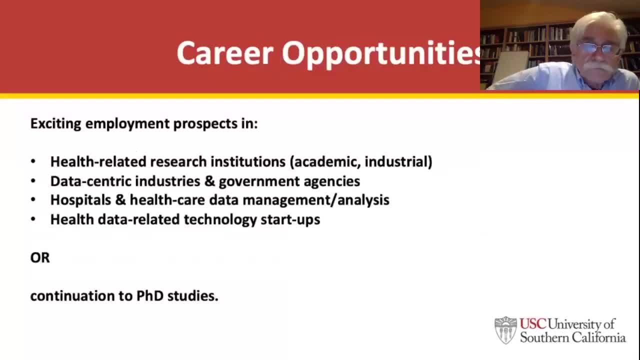 but more so and more importantly for you, it is a piece of evidence that in fact we are. we know what we're talking about when we talk about this particular topic. In terms of career opportunities, I believe there's exciting employment prospects, obviously. 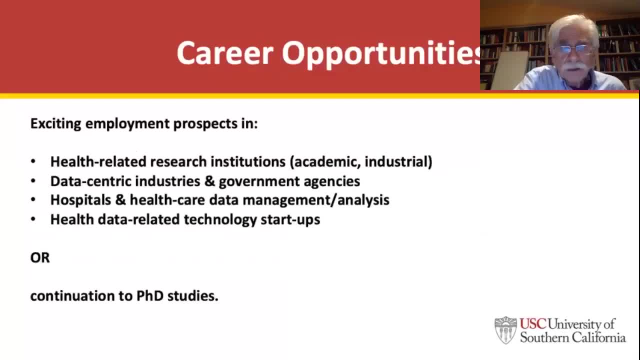 in health-related research institutions. this can be academic universities or it could be industrial. It could be also government, like NIH. It is also there are possibilities in what I call data-centric industries, which are many these days and continuously growing in number and strength, as well as government. 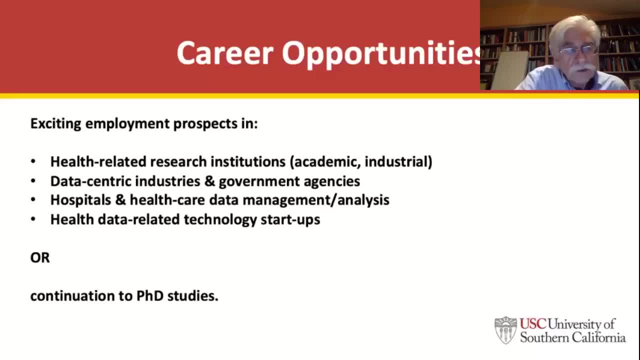 agencies. This could be, you know, CDC, or I guess one could put even NIH under that. Also, hospitals and healthcare data management analysis can utilize the skills more and more, And you know there's a lot of work to be done. 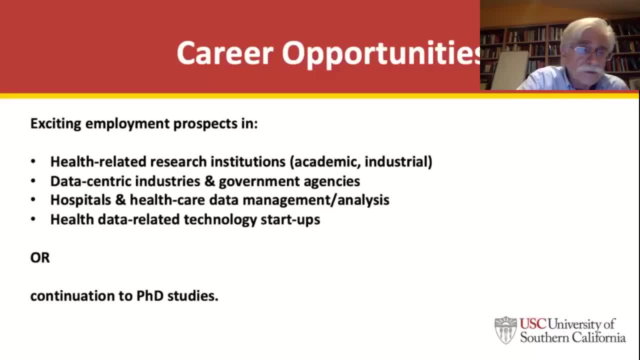 This last but not least, health data-related technology startups, which I think have a very bright future, And one of my sons is clearly interested in that, for instance, and I'm pleased to that he does so. In addition, of course, if you could use this as a springboard to continue on to PhD studies, 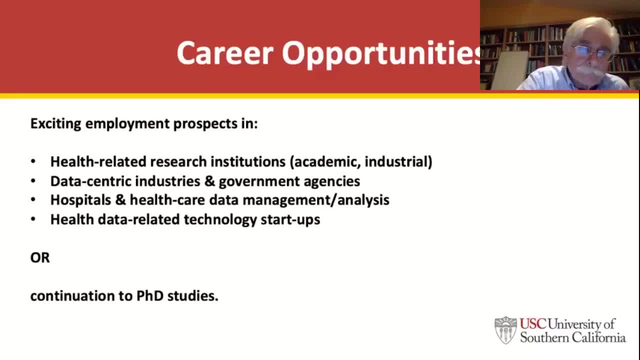 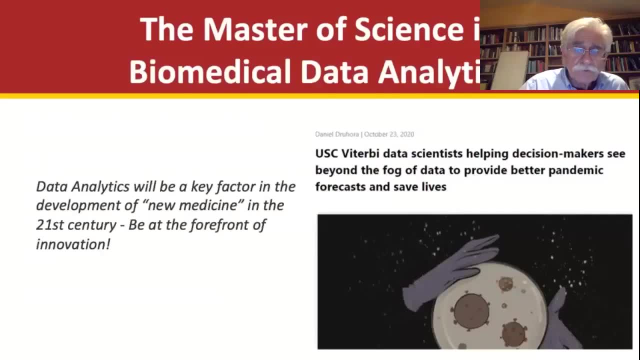 in a related subject. Let's see. a lot more can be said, but I will kind of limit my remarks to give you a chance to ask me questions. I think the quote we have on the left is I like it, I resonate with it- that data analytics. 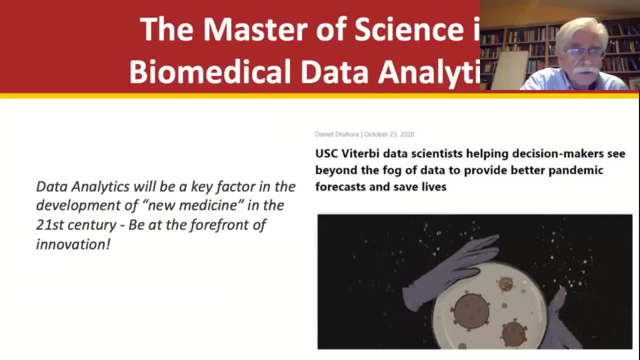 will be a key factor in the development of new medicine in the 21st century, And we'd like to be at the forefront of that, of such innovation. Now, this sounds grand, Grand And perhaps a little overreaching. I have no problem accepting that. 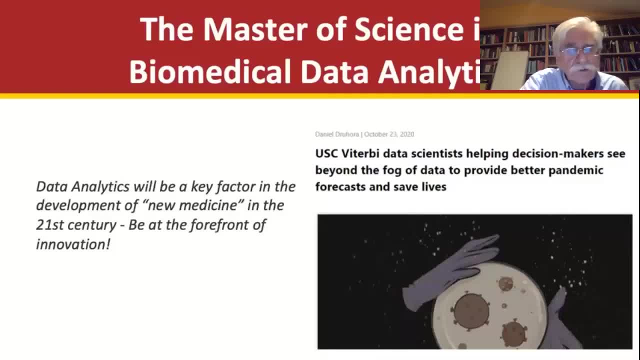 However, the essence of the statement is really valid and intact. If we are to transition into a new medicine, essentially we will have to rely on a much more sophisticated analysis of data that we may also, of course, acquire as well. It's not just first, we have to acquire them. 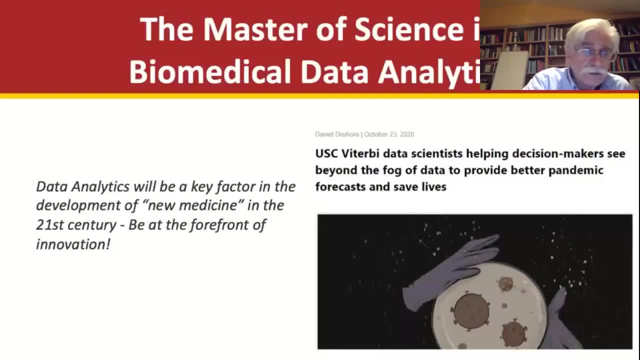 We analyze them, But both are needed. One cannot be without the other And it is my strong belief- and hopefully you will share that same belief- that the path to the new medicine that we all hope to have in your lifetime being much younger. 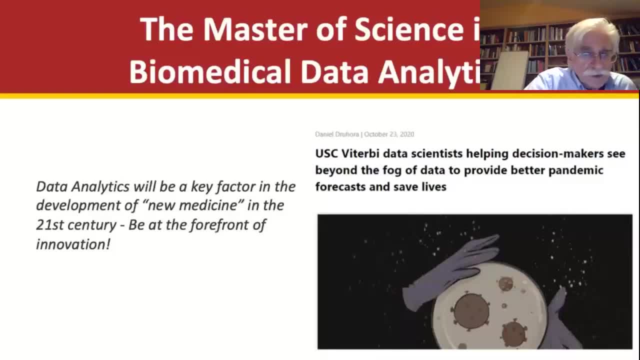 and I may not see it in my lifetime, but I hope your lifetime and my son's lifetime- you will see this And I hope the new medicine will benefit from this sophisticated analysis and do a much better job- yes, I would like to say a much better job- than we do now in terms 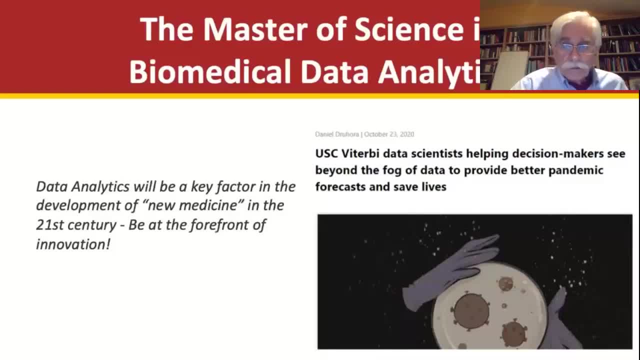 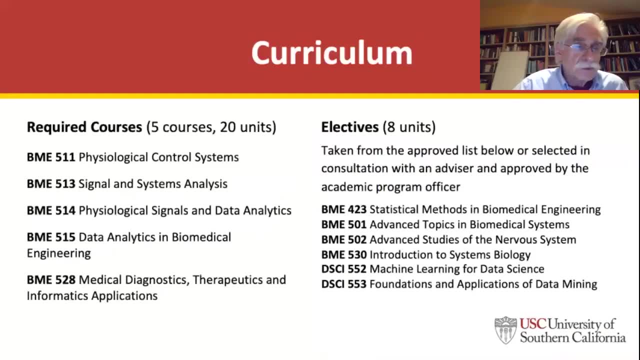 of healthcare. I will close the remarks by showing you the curriculum. I imagine you had a chance to look at the curriculum. I don't want to go down the list of courses but I could respond to questions if you have such. The titles are kind of self-explanatory. 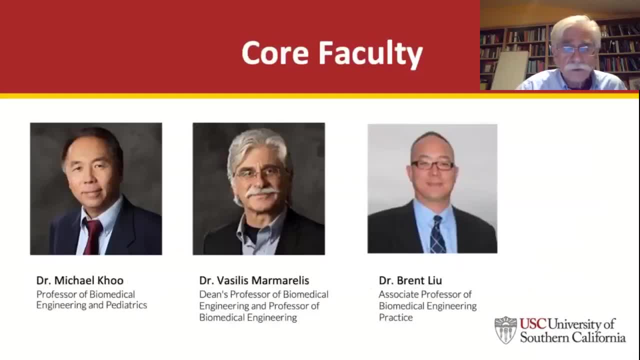 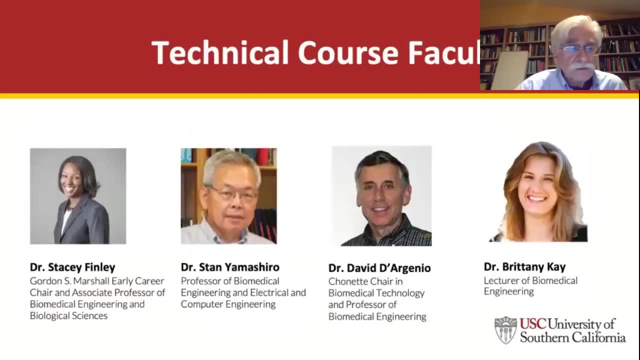 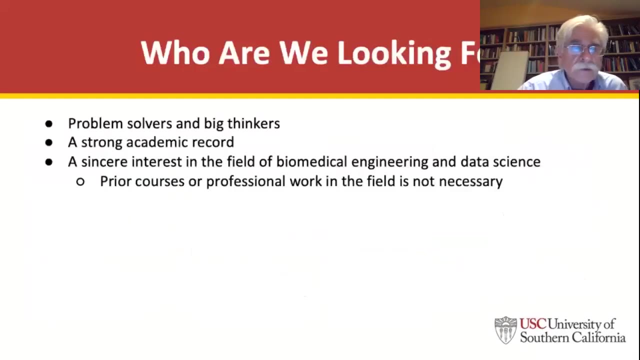 These are our faces: myself and my two colleagues who are contributing to this joint effort, And these are several of our colleagues who also participate in these classes. I would like to hear from you, if you feel like it, to tell me what brings you this evening. 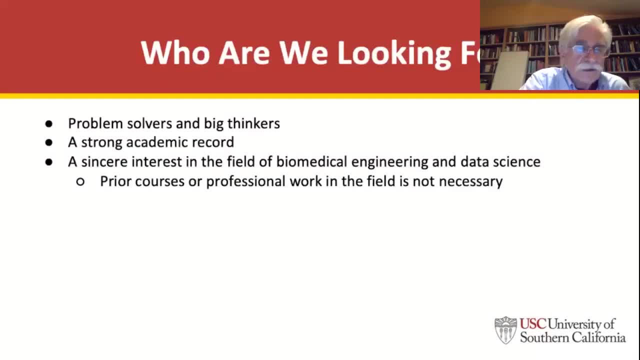 to this, whether you're into this and if you have any questions. but clearly we are looking for people who have active minds, like we all do have, and the problem solvers and we attract to big thinking. And also you must have a fairly strong academic record. 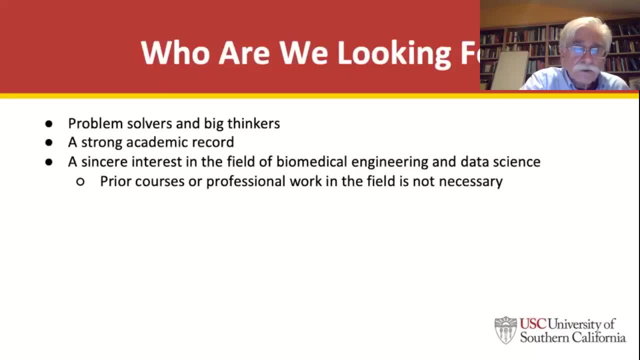 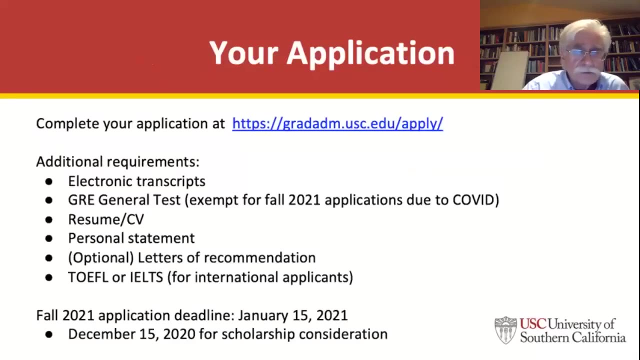 And clearly a strong and sincere interest in the field of bio-meta-engineering in the science. Yes, prior courses are not necessary. So I guess that completes the remarks, unless the host wants to say something on this. No, thank you so much, Dr Marmorellis. 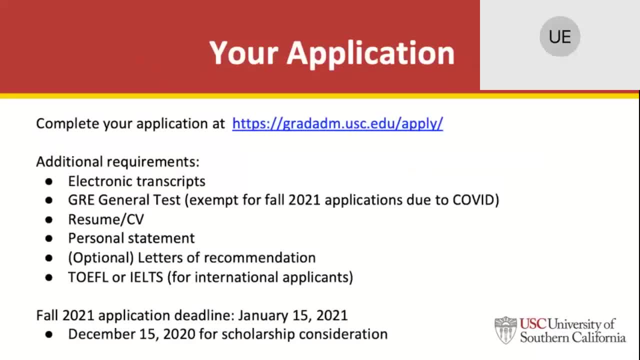 I would like to encourage our attendees: if you do have a question for Dr Marmorellis, please go ahead and ask in the Q&A box on your screen. So I'd appreciate it if you did that. And we did a quick survey prior Professor, just to gauge some of the panelists' background. 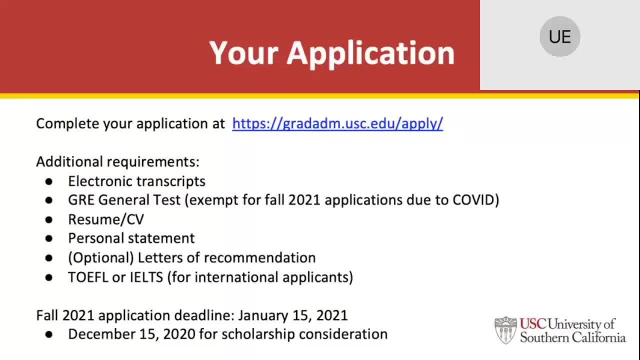 or the participants' background, And we had a BME, major bioengineering, major electrical engineering, signal processing, major People with those backgrounds I would imagine would be okay for a program like this. Correct, Okay, Go ahead. Wonderful. 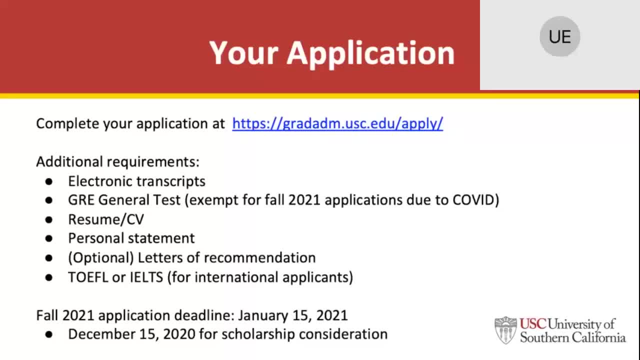 Okay. So yeah, please do start if you have any questions. I do want to mention that this upcoming cycle, fall 2021- applicants the GRE is actually being waived, due to you know, we try to be equitable in terms of people's access to the. 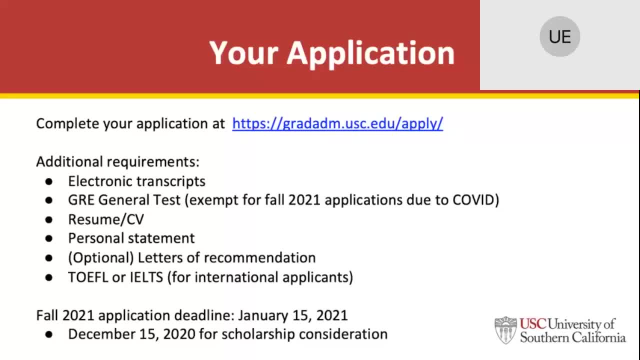 GREs with COVID and the pandemic. It may be difficult for some And not others, So we have decided to waive the GRE for fall 2021 applicants. I will need your help if there are actually questions, because I cannot monitor them on my. I don't see where I should be looking. if there are any, 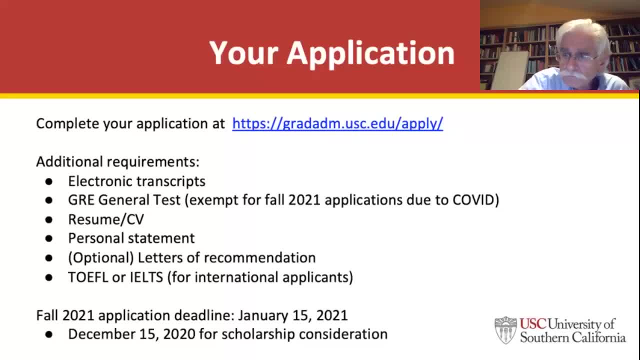 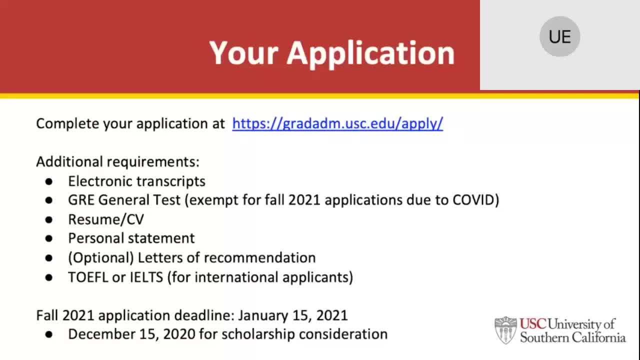 Let me see here Is there someone has asked a question about research. Is there a research component to this program? Perhaps you know this person claimed difference between a masters and PhD in a similar field. Are there research opportunities for this program? 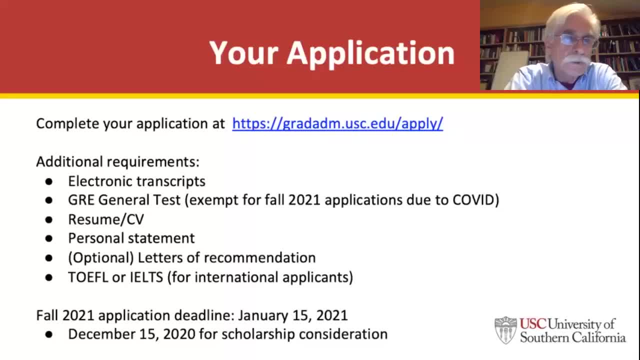 Yeah, That's a very good question actually. Yeah, And my brief answer is that, yes, there are opportunities that are not part at this point of the formal curriculum that we recommend. The reason is simply space in them, And I'm referring to units in the recommended curriculum. 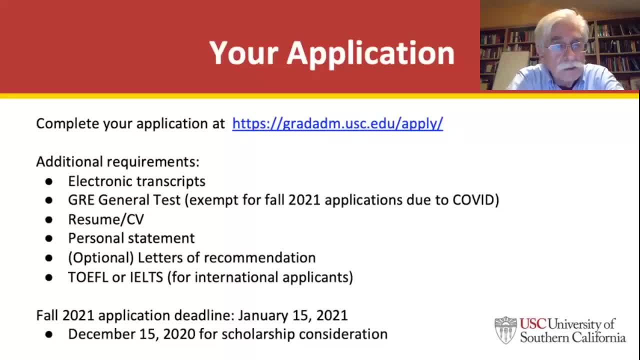 We do try to cover quite a bit of material And we could not put formally in directed research as a possibility of a certain number of units. However, I think our department and school has a tradition of being flexible to anything that's rational and makes sense. 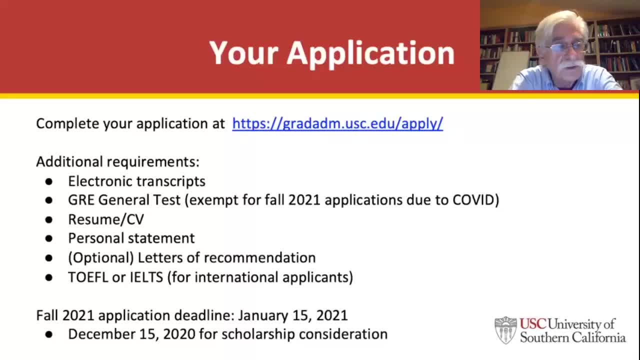 Therefore, if one has specific research interest and can work out with the proper person in the program an arrangement where this person can take directed research for a certain number of units instead of a single class, So that can be accommodated if such interest exists. 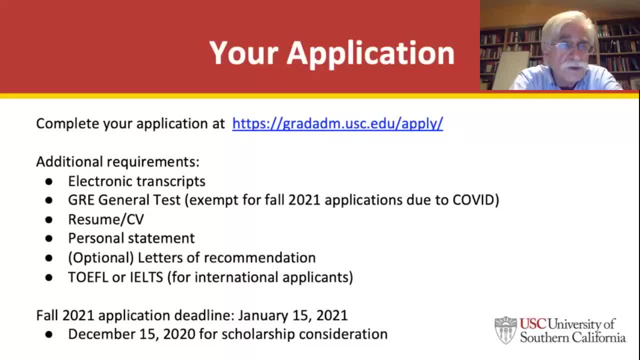 But normally this is rather course intensive program. Excellent, Thank you. Thank you for that, Let's see. I have another question. Let me see What are the differences. I'm not sure we'll be able to answer it. What are the differences between this program and a concentration of biomedical engineering? 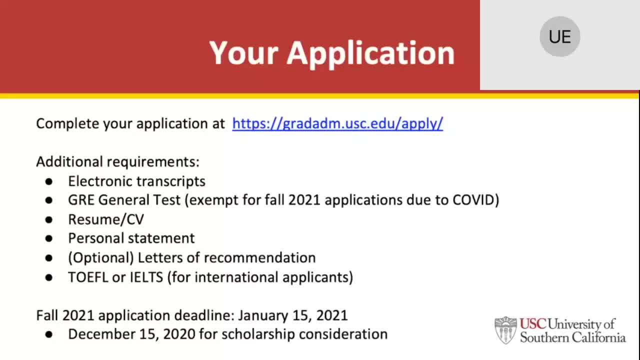 and electrical engineering. We actually don't have a concentration of biomedical engineering, Okay, So I'm not sure if you can talk about that. I mean, I would say we have a concentration of biomedical engineering and electrical engineering within our electrical engineering department. 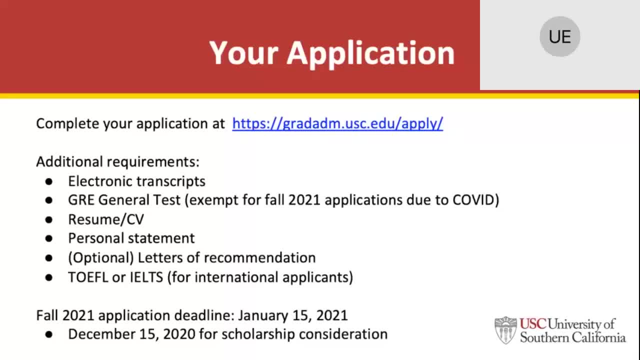 So I'm not sure about that one. Someone's asking if there is research dedicated to brain computer interface. I'm not sure within biomedical data analytics. if there is, I'd imagine not, But I will ask you if you. The question was about BCI- brain computer interface. 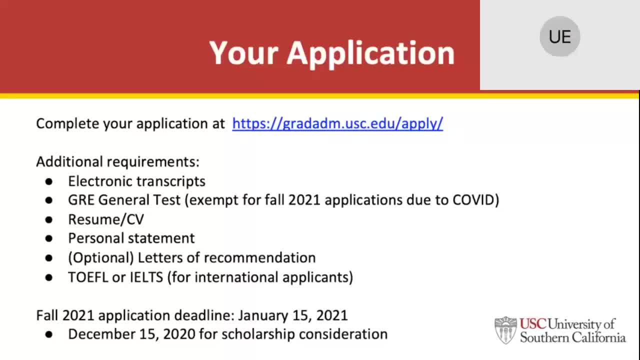 Correct, Correct. Yes, It's an area that we have had quite a bit of presence in terms of the research over the years, primarily through the work of my colleague, Ted Berger and his associates and myself and my lab. Other people as well have done work in our department, of course. 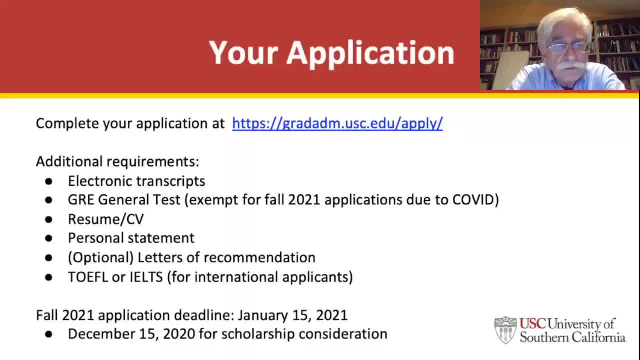 But obviously I'm most familiar with the work, the research I just mentioned. So we have done quite a bit on that. But at this point that area of research is active but not in a big way the way I see, at least from my vantage point. 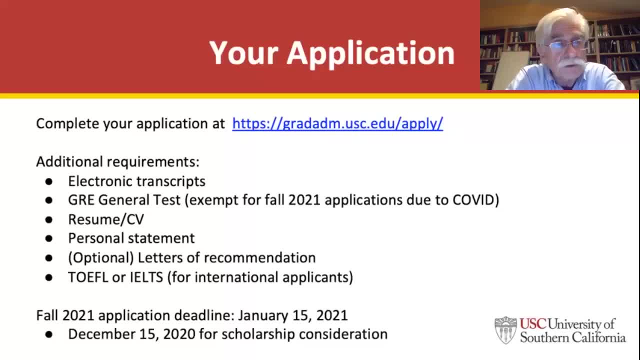 There are people. There are people in the School of Engineering who are interested in BCI and do have active research programs, But I will have to defer to them for more specifics. I would not. What this program may offer to the BCI is simply some methodologies to analyze the data. 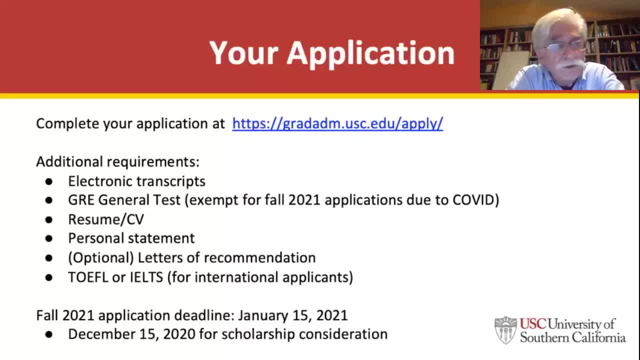 collected through those brain and computer interfaces. Great, I had a question From the audience, From an attendee. How does this program approach or take advantage of time series data coming from common wearables like Fitbit or the Oura Ring? Yeah, 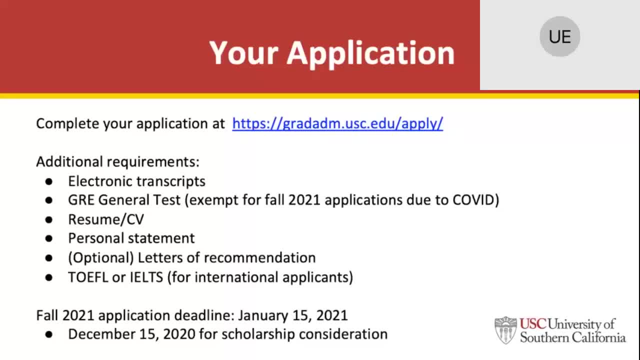 Very much. The brief answer is very much, so I'm trying to choose my words so that they don't take too long. You know professors like to talk a lot, So I'll be careful with this. This is late in the evening for all of us. 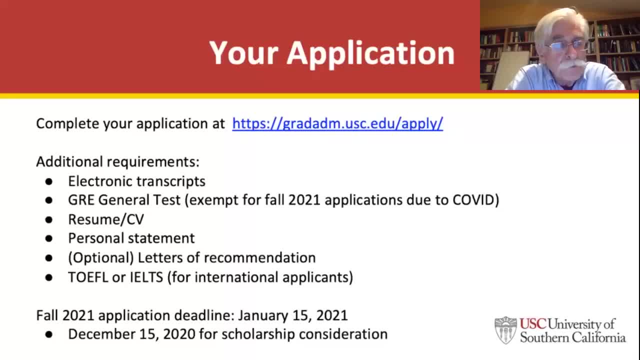 But I'm trying to choose my words so that they don't take too long. You know, professors like to talk a lot, So I'll be careful with this. This is great, Definitely. my answer is definitely strongly affirmative. In other words, we can. I would like to see one of them, as I already indicated, one of. 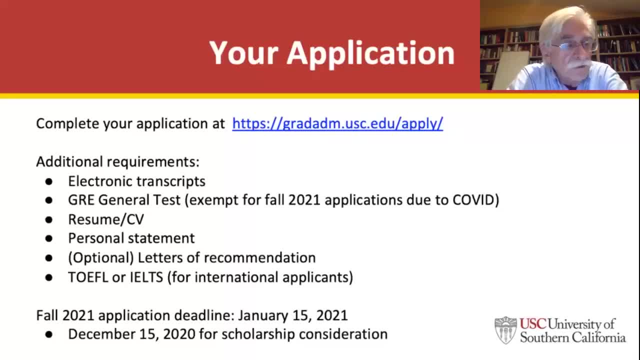 my sons has such an interest and I certainly encourage it And I follow great interest. obviously I myself have an interest in that, But competing with others. But again, the answer is absolutely yes And I would like to see more data. 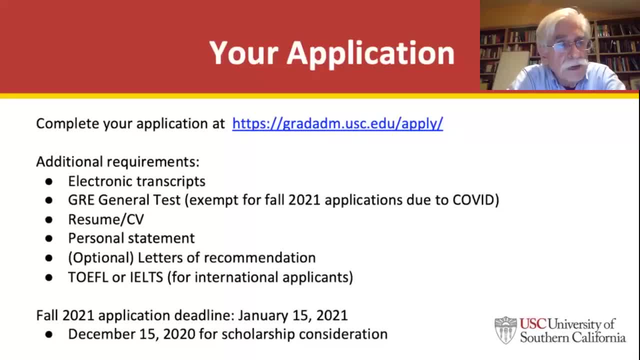 Thank you. I'm curious to see more young, ambitious, driven, highly intelligent people like you be involved with that. Yes, absolutely. I gave an example of that. It was a simple example by necessity, But you know you can imagine it's a lot more one can do with blood pressure. 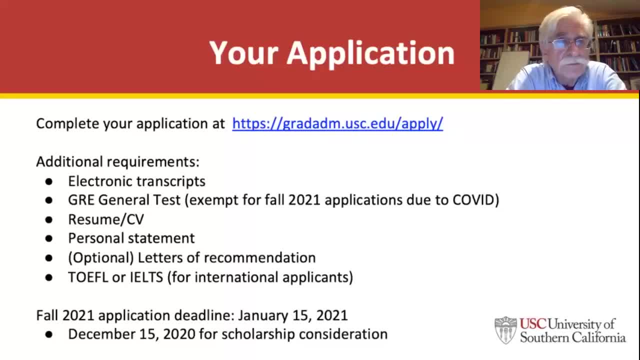 I'm talking about things that you can easily measure these days side of heart rate and oxygenation, And, you know, I would love to think that this will become more sophisticated. more sophisticated, we develop also sensors that will give us access to more wearable data. 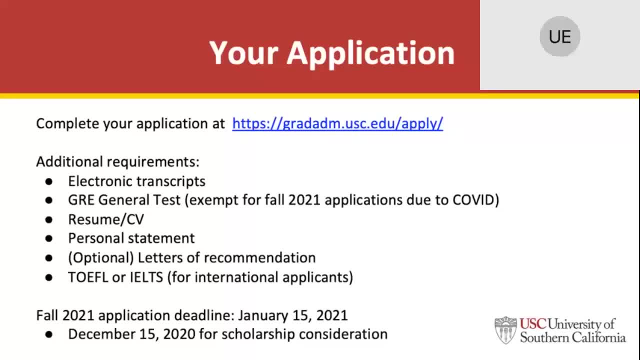 Thank you so much. Does anyone have any additional questions for Dr Mamourelis? Okay, Well, if there are no more questions, I just want to remind everyone about our application deadline. The deadline is listed on the slide here. We do have an earlier application deadline. 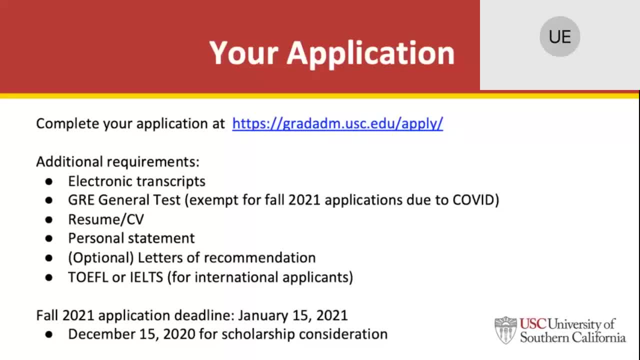 of December 15th for scholarship consideration and we do have a limited number of merit-based awards that are partial scholarships. If you apply by the December 15th deadline, submit your online application and transcripts. They just need to be original transcripts, scanned and uploaded into the application portal. 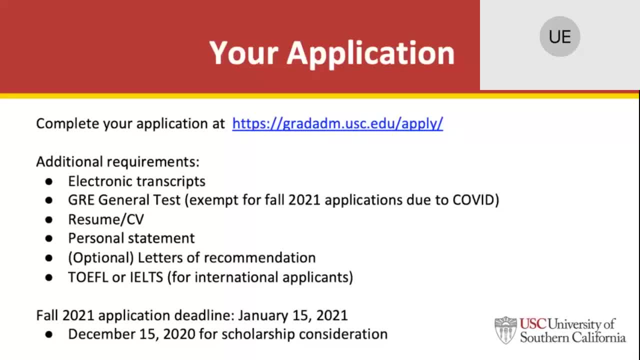 Then you'll be considered. if you're admitted, you'll be considered for these scholarships. There's an interview process as well. in regards to that, Our final application deadline is January 15th of next year. so just know the two distinctions between that. I did have another question. come in. 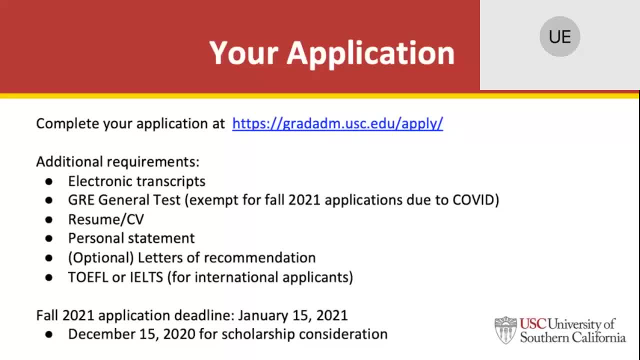 while I was talking about the application deadline. The application deadline is January 15th of next year, so just know the two distinctions between that. I did have another question come in while I was talking about the application deadlines, asking: what computer languages or software does the program focus on? 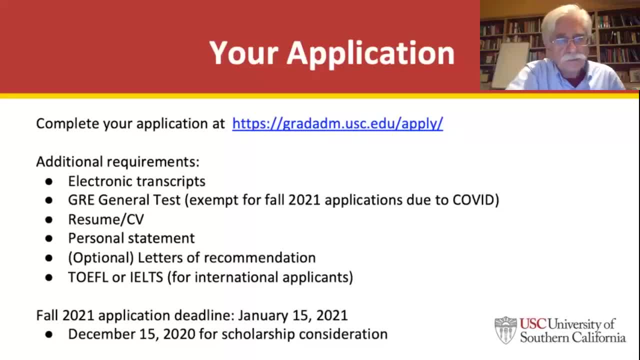 We mostly use actually MATLAB because it has become quite a standard in our particular field of system modeling, data and other signal processing et cetera. But I really don't want to rule out other possibilities that one can use other types of popular computer languages these days to write these programs. 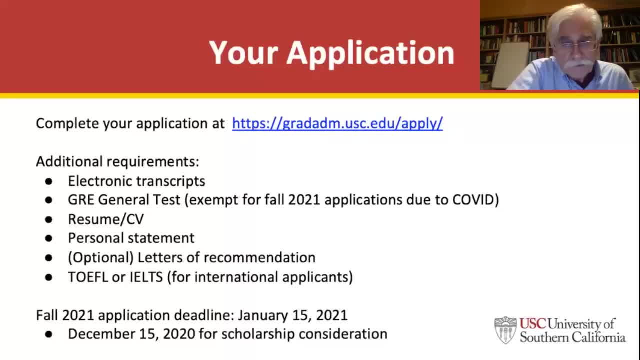 So I would leave that open, but in terms of instruction and part of the courses, I would expect that MATLAB will be the software language that will be used primarily. Thank you, But I should note that you understand my limitations in speaking on behalf of my 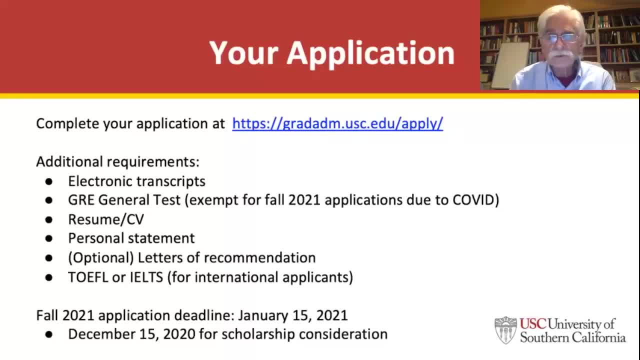 colleagues who teach their courses, because I do not tell them what to teach exactly. We agree to teach specific, particular topics and a general outline, but of course the responsibility for the specifics are up to each instructor, as you understand. So this answer of mine primarily concerns the courses that I will be teaching, which is two of the courses using the curriculum. 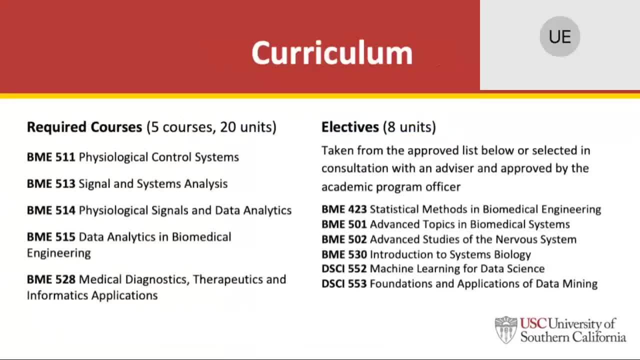 Yes, and it just looks like just going over that briefly, there are five required courses and then two electives, I believe eight units that the student can select from. So there's a little bit of flexibility for a student to choose and select.